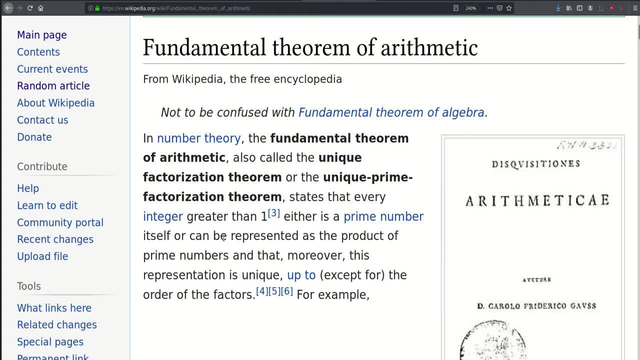 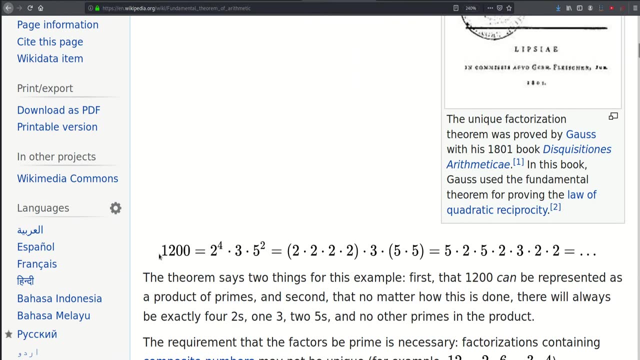 greater than one either is a prime number itself or can be represented as a product of prime numbers, And that, moreover, this representation is unique And that's very important. So, given any number- like here, 1200,, we can represent this as 2 raised to the fourth power times 3 times 5. 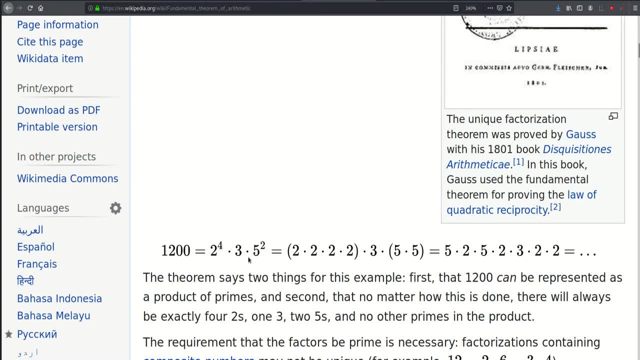 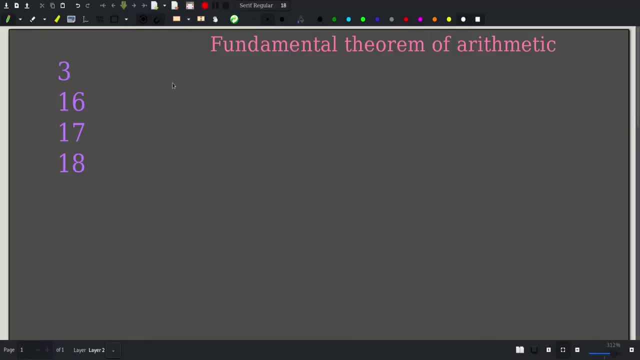 squared And if we order the prime factors in increase on order, this representation is unique, So let's go ahead and factor our numbers in this manner. So this will be equal to 2 raised to the fourth power, 17 is a prime number, so it would be just equal to 17.. And 18 is 2. 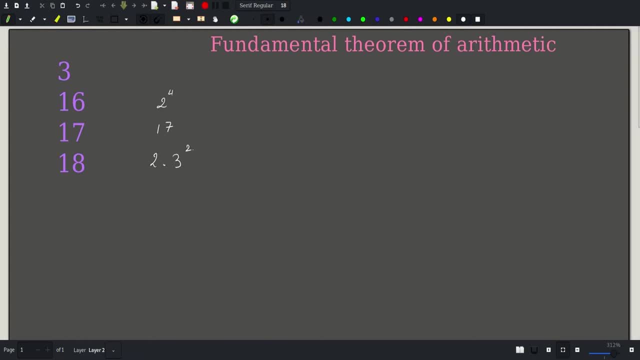 times 9.. So 2 times 3 raised to the second power. Great, Now we want to find the number of divisors of 16.. Okay, So let me ask you a question: Can 3 be a divisor of 16?? And the answer is no, because 3 does not show up. So let's go ahead and find the number of divisors of 16.. And the answer is no, because 3 does not show up. So let's go ahead and find the number of divisors of 16.. And the answer: 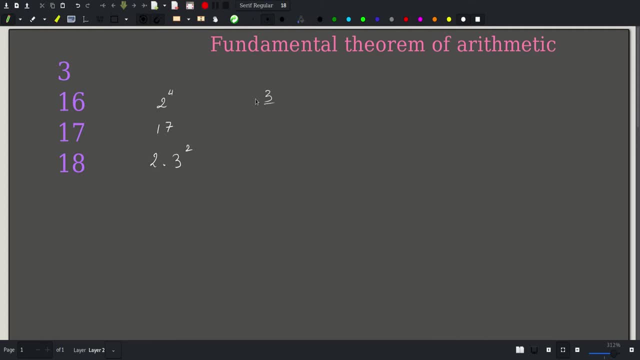 is no, because 3 does not show up. So let's go ahead and find the number of divisors of 16.. In other words, any divisor of 16 has to belong to this list, And since 2 is the only prime factor, 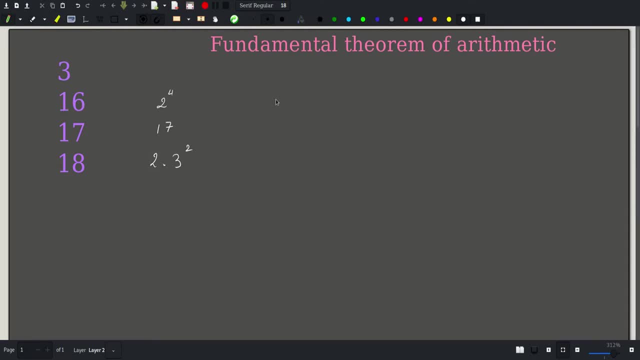 of 16, then any divisor I come up with can only contain 2.. And the second question I would ask you: can 2, raised to the seventh power, for example, be a divisor of 16?? And the answer is again, no. 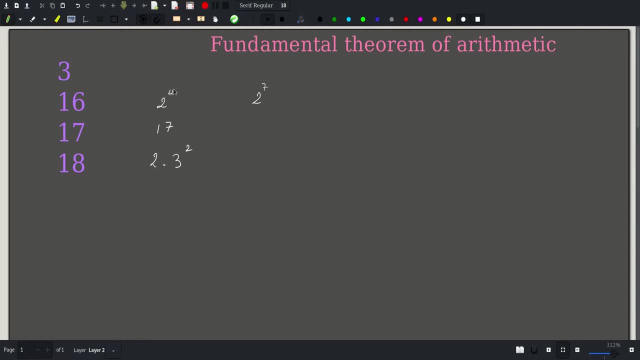 because 16 is equal to 2 to the fourth, And thus the largest power a divisor of 16 can have is 4.. So basically, all divisors of 16 would be of the form 2 raised to some alpha, And alpha is between: 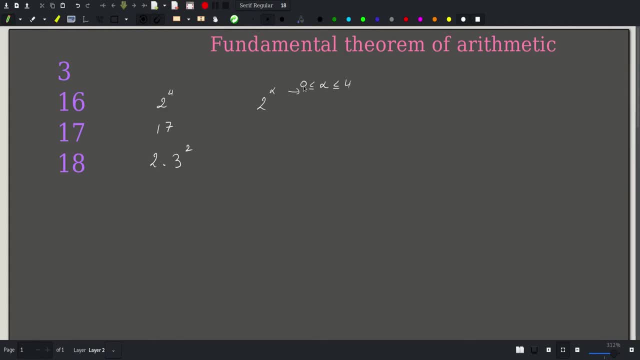 0 and 4 included, It can be equal to 0. And that's the case where the divisor is equal to 1.. 1 is in, indeed, a divisor of 16, and it can be represented as 2 raised to the 0th power and the maximum. 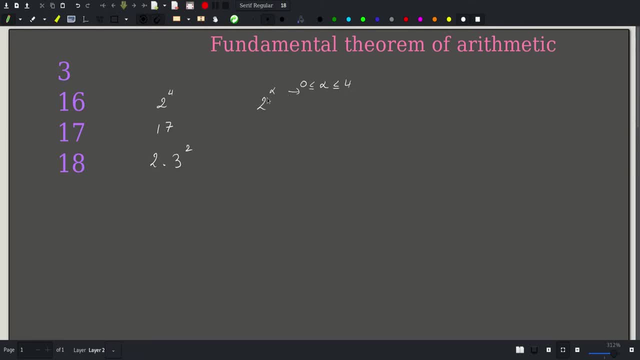 value alpha can take is 4.. So basically, 16 will have 5 divisors, that are, 2 raised to the 0,, 2 to the 1,, 2 to the 2nd power, 2 to the 3rd and 2 to the 4th and it won't have 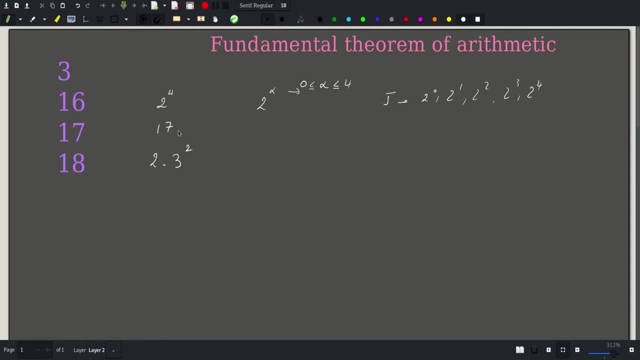 any other divisor, The same goes for 17.. So all the divisors of 17 can only contain 17, and the alpha here is between 0 and 1, because here it's topped by 1, and therefore the number of divisors for 17 will be just 2,, namely 1 and 17.. What about 18? now Our divisors. 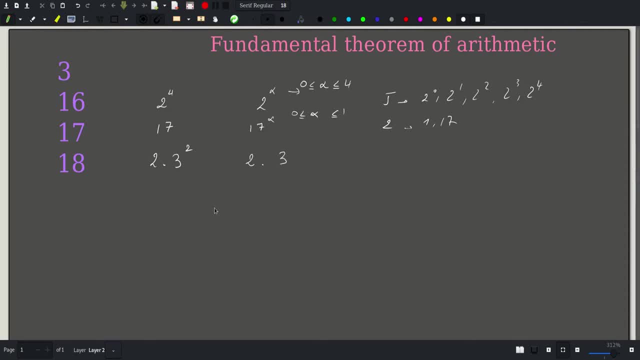 can either contain A2. Or A3. We have a choice here, And we have 2 powers here: alpha and beta. And alpha here can be anything between 0 and 1, whereas beta can be anything between 0 and 2.. So here we. 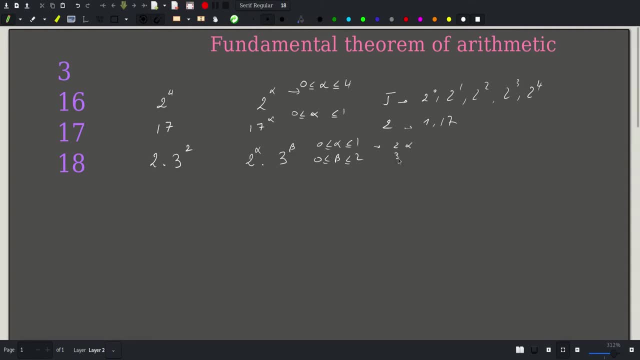 have 2 choices for alpha and 3 choices for beta, And since our choice of alpha is independent of our choice of beta, Then we have 2 choices for alpha and 3 choices for beta, And since our choice of alpha is independent of our choice of beta, Then the total number of possibilities will be just. 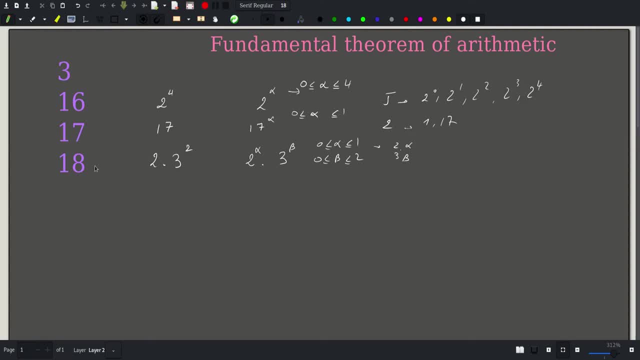 the product of these two, And consequently, 18 will have 2 times 3, which is equal to 16.. And consequently, 18 will have 2 times 3, which is equal to 6 divisors. And these are all the combinations of 2 raised to some alpha times, 3 raised to some beta, where these are. 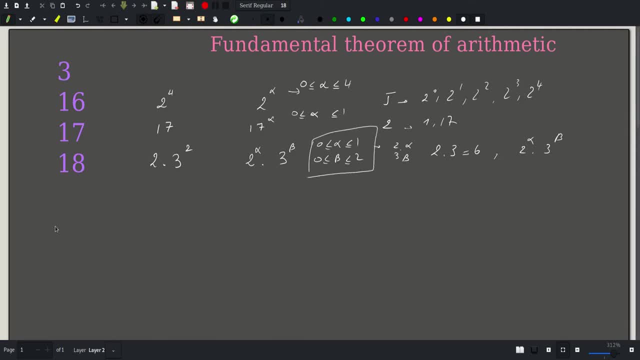 the constraints on alpha and beta. So, in general, any number x that is equal to p1 raised to the alpha 1 times p2 raised to the alpha 2 times p3 raised to the alpha, 3 times pn raised to the alpha 1, has a number 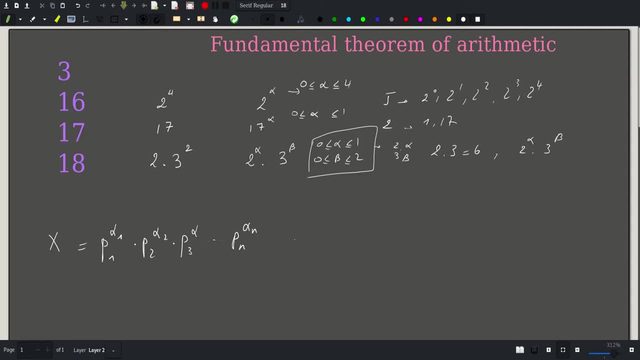 of divisors. that is equal to the product. So this is equal to the product. We represent the product with pi here, as we represent the sum with sigma. So this is equal to the product. from i equals 1 to n of alpha, i plus 1. And we have a plus. 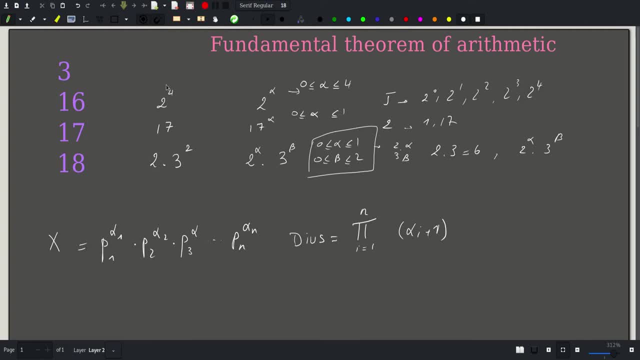 1 here to account for the 0. So remember like here we had 4 and we had 5 divisors, because 5 is equal to 4 plus 1.. So basically, this alpha i plus 1 represents our choices for alpha 1.. 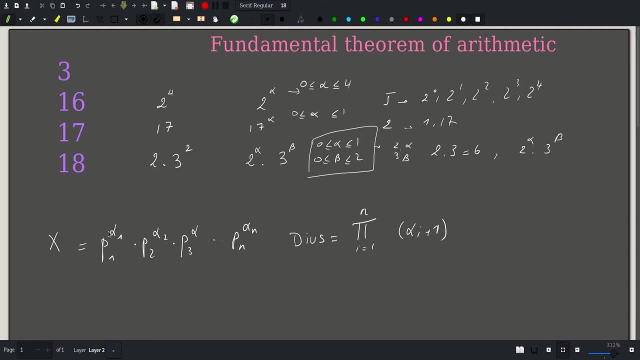 So for alpha 1, for example, we can have 0,, 1,, 2,, 3 up to alpha 1.. So the total number of choices is alpha i plus 1. And that's pretty much it. Our number of divisors will be just equal to this product. 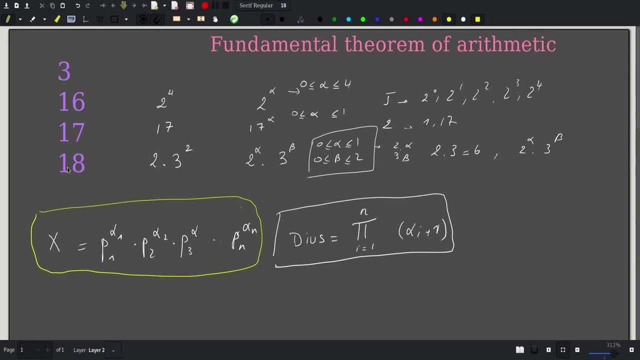 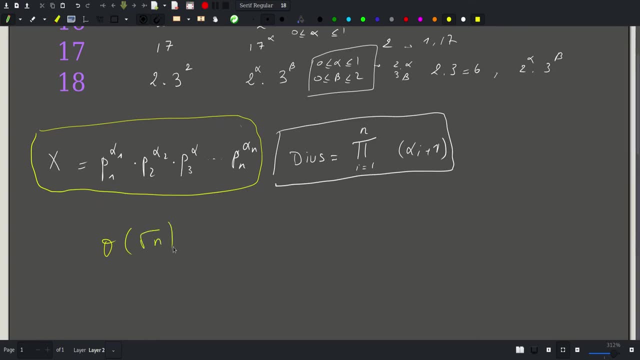 And now all what is left is to find this factorization for the numbers that we will be given And, as you may know, there is an algorithm that runs in all of square root of n, that finds all the factors of any given number. So, basically, all what we have to do is go from i equals 2 up to square root of n, i less. 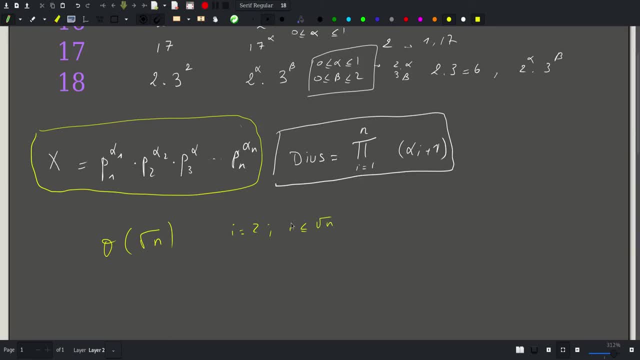 than or equal to the square root of n, And actually we don't use this comparison because taking the square root of n requires the use of some function that takes the square root of n, And introducing this may lead to precision issues. So instead we check that i squared. 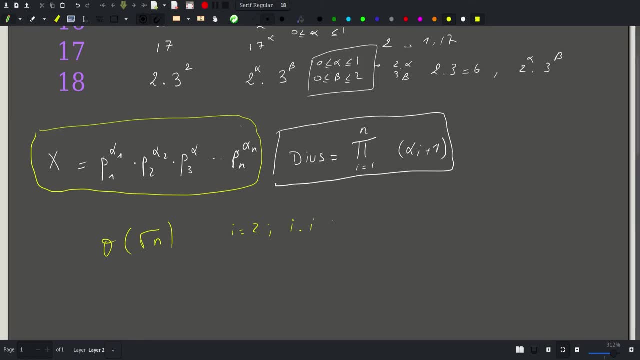 is less than or equal to n. So i times i is less than or equal to n, i plus plus. And for each value of i we check if n modulo i is equal to 0. That is, i divides n And if that's the case we will just keep dividing. So while n modulo i is equal to 0, we will. 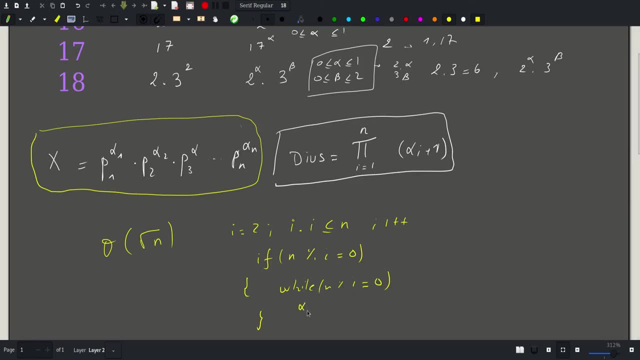 keep dividing n by i, And each time we will increment alpha. So that's it. So alpha plus plus Alpha here, representing our power- And at the same time we will divide n by i, And after we do this, we just record this value of alpha and that's all what we're going to. 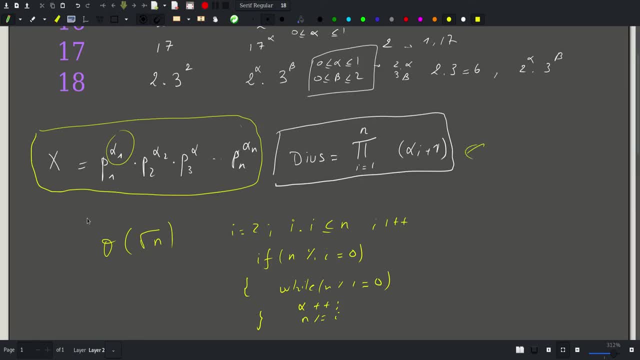 require in our problem here. But we can also record this pair, that is, the prime number, along with its exponent if we want to retrieve the whole factorization. But in our problem here all what we are interested in is these value of alpha. So we will require all of √n for finding this factorization And for this computation. 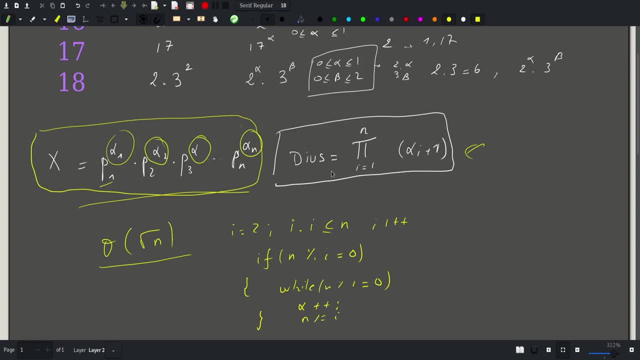 here for finding the product of the alphas in order to find our answer. this one requires that much computation Because the worst case is that our number is composite, That is, it contains many prime numbers, And this is the result that we get, Because alpha x equals. 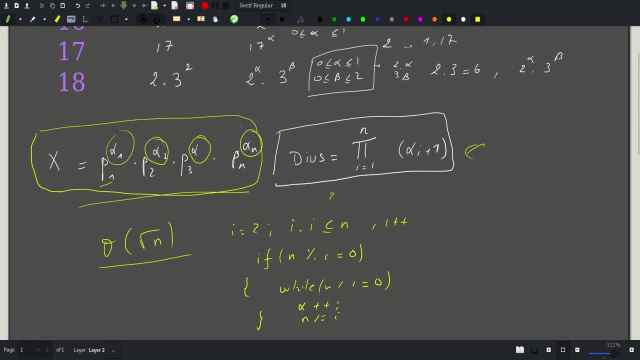 alpha plus minus this, And it contains many prime numbers And that shouldn't taste better. So we said we need to physique this. If we can do it in the other way, then we'll make is that our number looks something like 2 times 3 times, 5 times, 7 times 11 and. 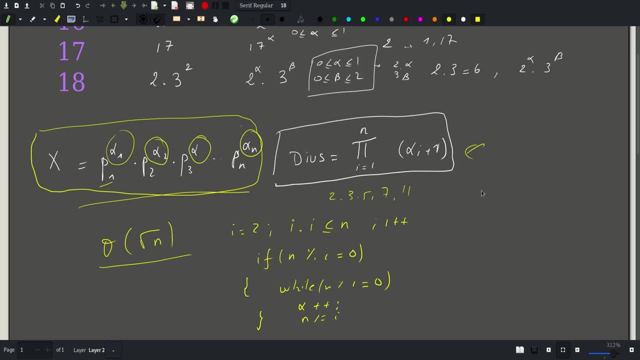 so on, and since our number can be only as large as a million, this can have at most a few prime factors. so here, if we add a few more, we can see that having 10 or up to 20 is gonna go beyond 10 to the 6 pretty quickly. so here we gonna. 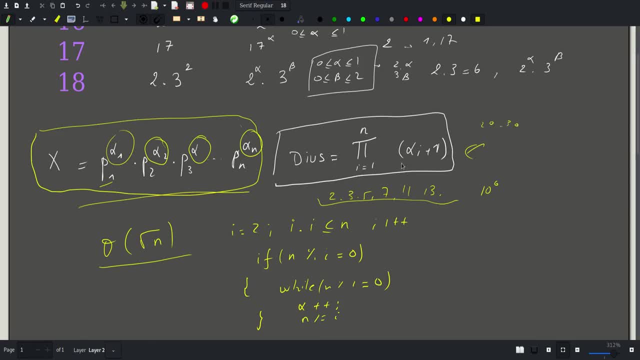 perform at most 20 to 30 multiplications. so this won't account much for the, for computing the complex, for for our complexity. so our total complexity will be square root of n plus whatever this is. so let's say 30 plus, and all these times the number of queries we have here, which can be up to. 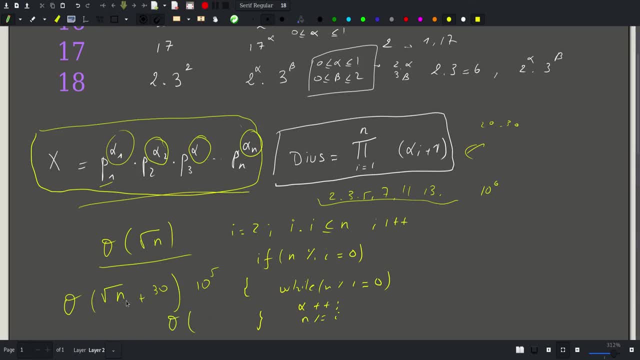 10 to the 5th. so our total complexity here will be 10 to the 5th. so our total complexity here will be 10 to the 5th. so our total complexity here will be 10 to the 5th, 10 to the third times 10 to the fifth, which is about 10 to the eighth. 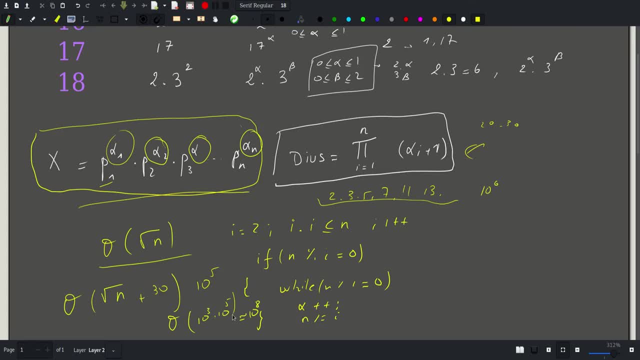 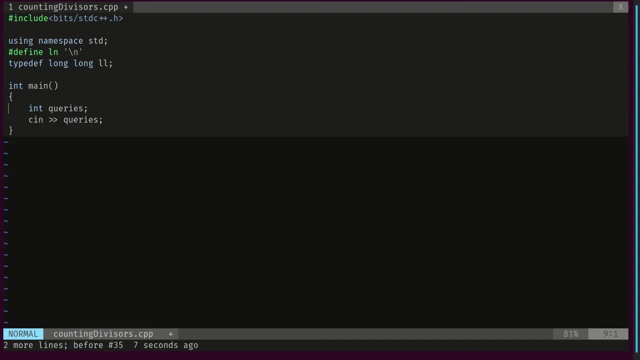 And this is within our threshold, so we are fine. Now let's check out our code. So this is our program. We will start by reading the number of queries we will have to answer, Then we will process them And for each query we will read our number. 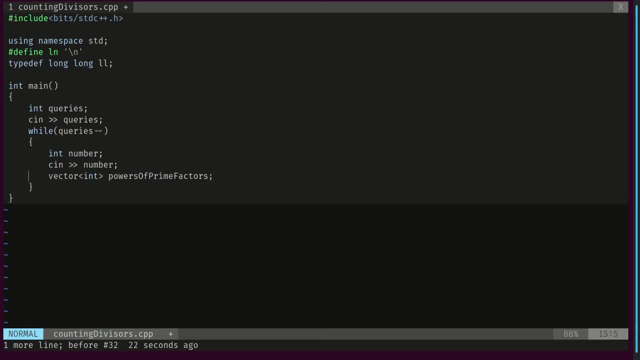 And for each number we will declare a vector of int that will store the alphas that we mentioned, So it's going to store the powers of prime factors. Then we're going to factorize our number. So, as we said, we're going to have a for loop that goes from 2 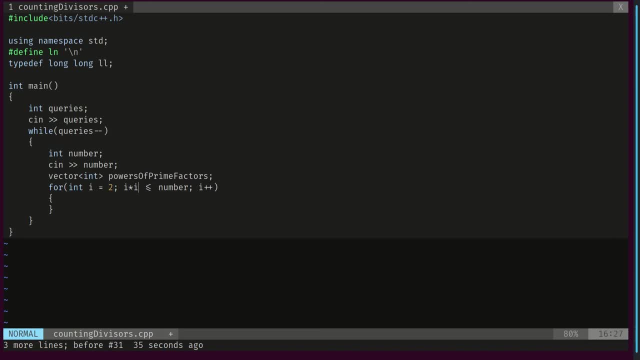 up to the square root of our number And we'll check for this by checking that i square is less than or equal to our number. And each time we're going to check if the number is divisible by i, That is the number. modulo i is equal to 0.. 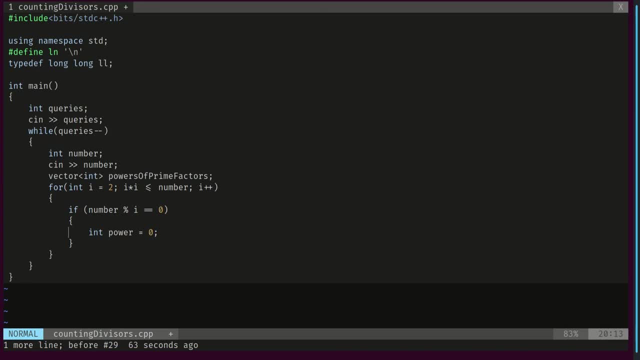 And if that's the case, we're going to declare our power that we're going to keep incrementing And while the number is divisible by i, we're going to increment our power and divide the number by i And at the end we'll just push this power into our vector. 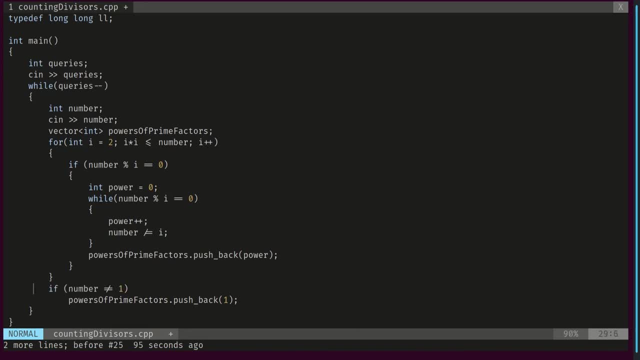 And when we are done, we might have that the number is different from 1.. So, for example, say that the number here is 17.. 17 is not divisible by any number that is smaller than it or that is different than it, because it is a prime number. 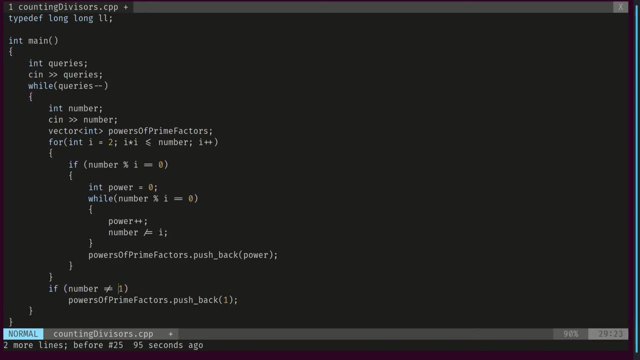 So at the end here we're going to have, that number is different from 1. And that's why we have to push 1 into our vector, because it accounts for the power of 17 in the prime factorization of 17.. Whereas if we had some composite number here, like, let's say, 4,. 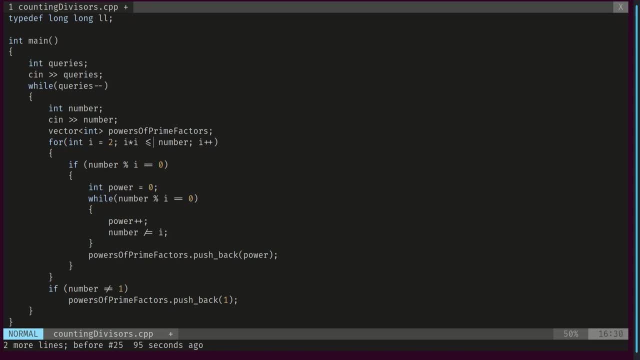 we're going to start with 2.. And 2 times 2 is less than or equal to 1.. 2 times 2 is less than or equal to 1.. 2 times 2 is less than or equal to 4.. 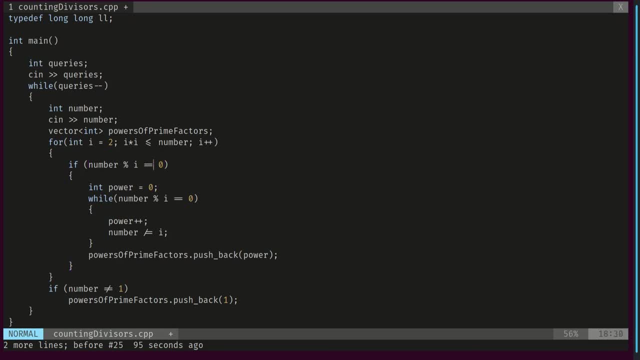 And we're going to find that 4 modulo 2 is indeed equal to 0.. So we're going to initialize our power with 0. And then, while 4 is divisible by 2, then we're going to increment our power once and divide 4 by 2 to get 2.. 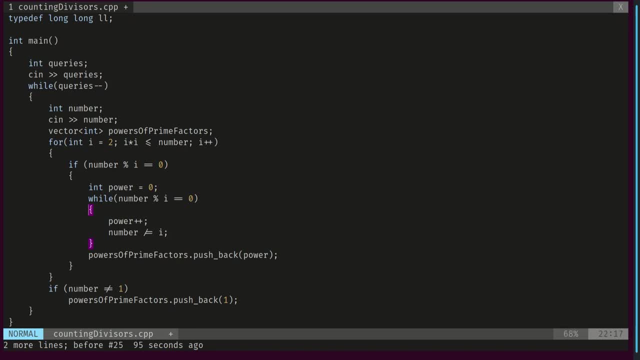 And then again we're going to have that 2 is divisible by 2.. So we're going to increment our power a second time and divide number by 2. And this time the number is equal to 1.. So when we get to this point,